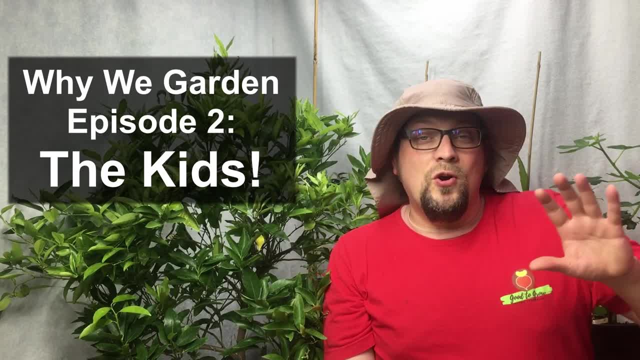 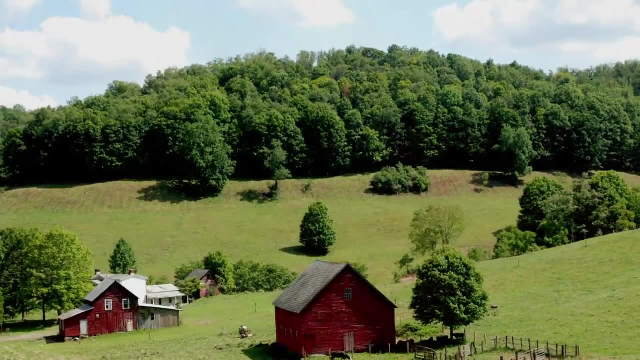 children. So my personal recollection. as early as I can remember, you know, I grew up on a farm until I was about five or six years old. That was a 300 acre farm, and while there were quite a few animals on that farm, I distinctly remember some really nice garden plots as well, and I have lots of 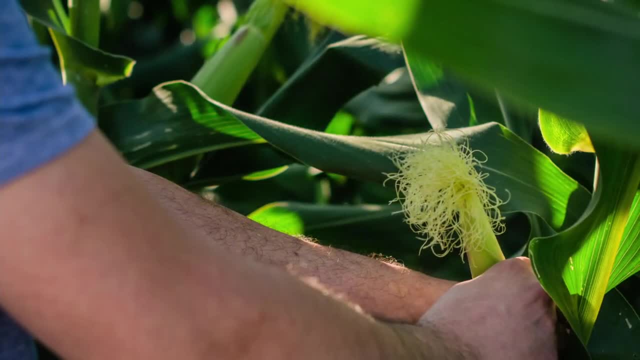 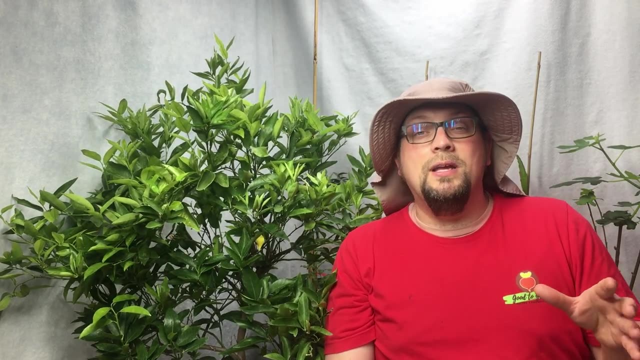 great memories of going out picking beans and corn and tomatoes and all of those really nice healthy, organic, fresh vegetables. You know, and while one side of my family had a farm that they lived on, the other side of the family didn't have a farm but they definitely had gardens. 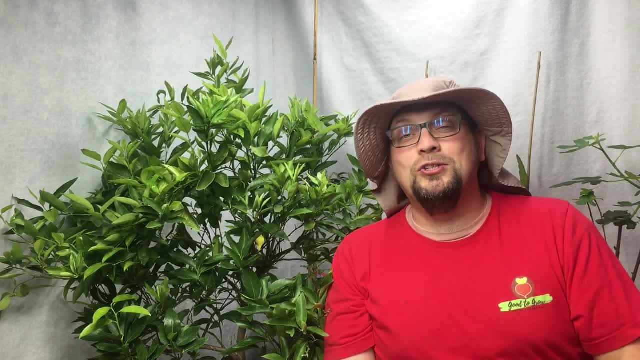 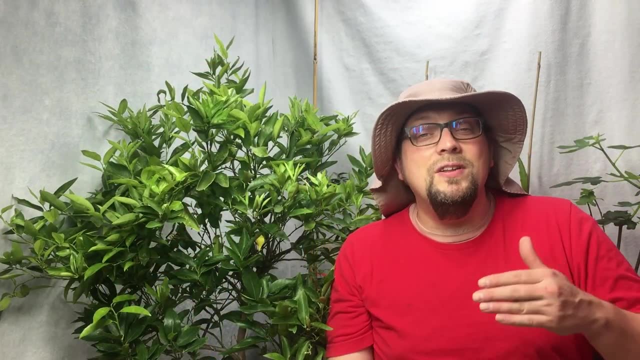 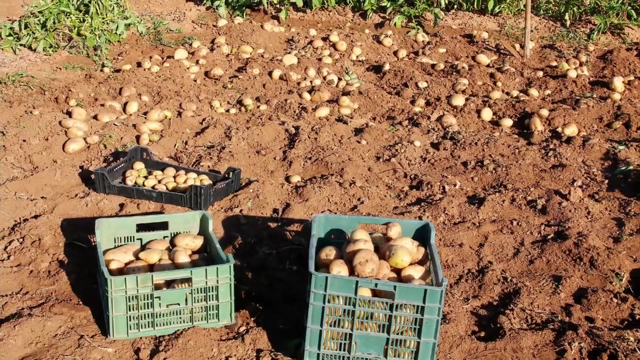 and there was a real canning culture. I guess I would say There were so many things that we had that were canned, that we were preserving, and I have very clear memories, even as young as five or six years old, of spending time with my grandmother out in her garden area, both planting, 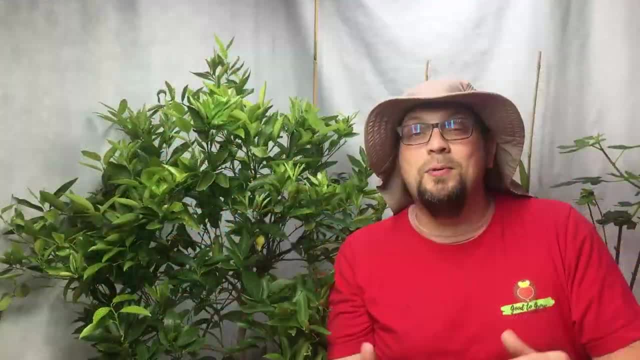 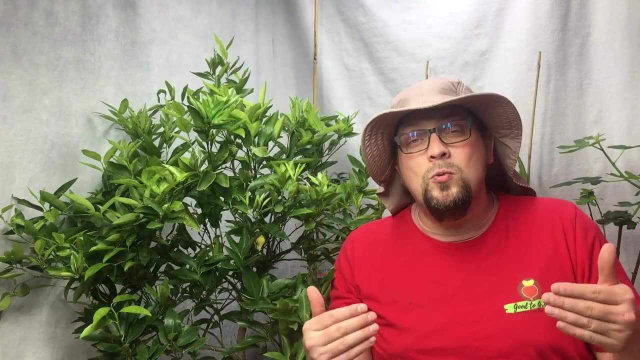 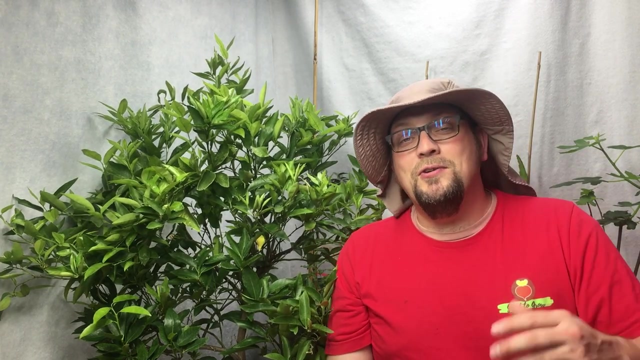 and then harvesting. She had been growing potatoes- and what can I say? potatoes have been with us for a long time. and also she had a really, really nice strawberry patch. Those memories stick with us because that's a part of who we are growing up Now. is that the same for everyone's experience? I don't know. that's. 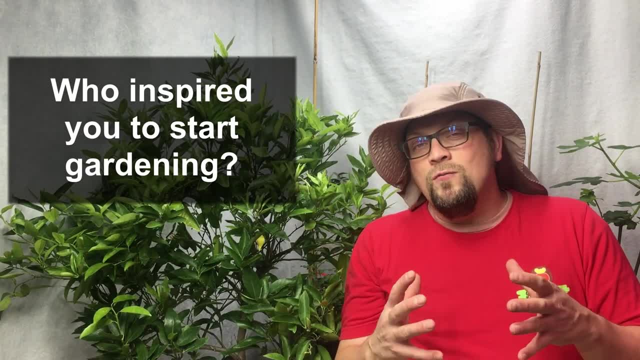 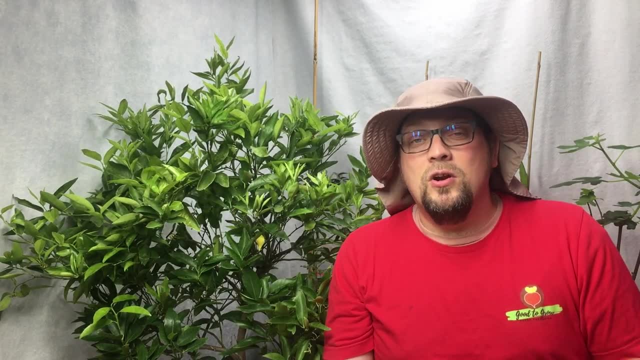 why I want to hear from your comments in the description. A big part of what we're doing here in terms of gardening and why we want to garden, has to do with our children. Now, there are a lot of things that we can do to encourage our children to be a part of our gardening experience. 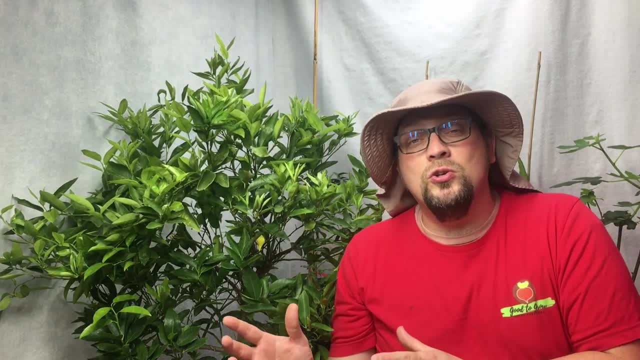 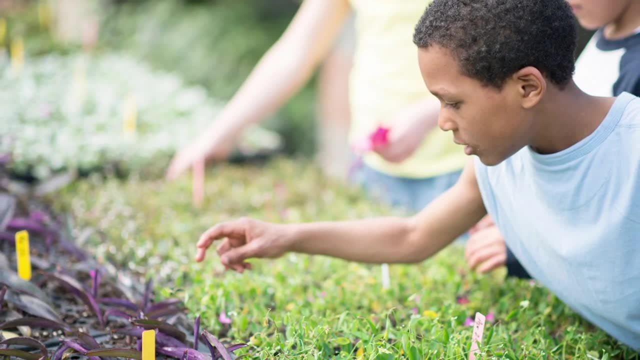 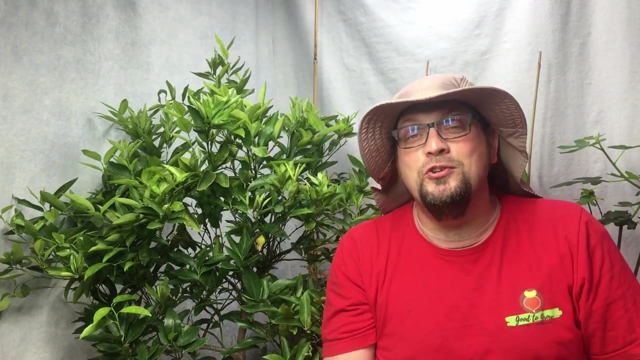 but one thing I can tell you for sure: the benefits of having children exposed to gardening are so profound and so clear that it's really, in our opinion, a no-brainer when it comes to getting our entire family involved. Now, if you've been watching our content on this channel, you know that we 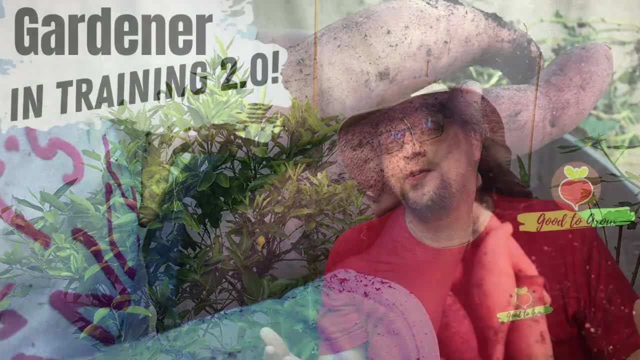 actually have an entire playlist dedicated to our Yardners in training. That would be our daughters who will help us out with different harvests and all that kind of stuff. So if you're interested in gardening and you want to learn more about gardening and how to get involved with gardening, 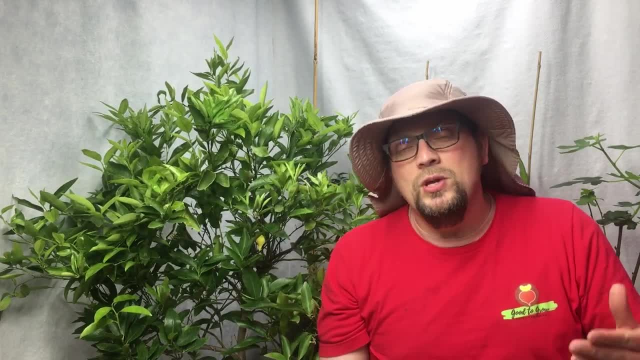 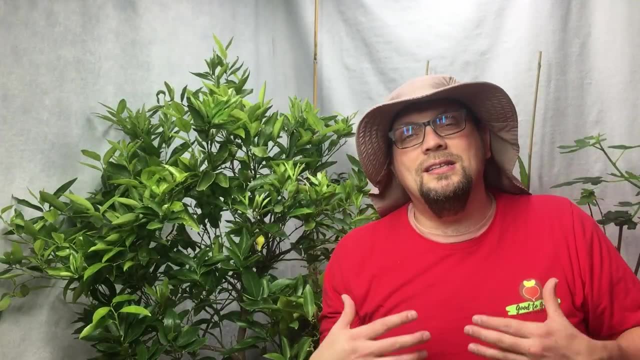 also with their explanations of what's going on. we even did a nice tour led by our youngest Yardner in training earlier this season. So we get them out there, we get them involved in this process of gardening and what we see is not only that, they're learning and picking up information. 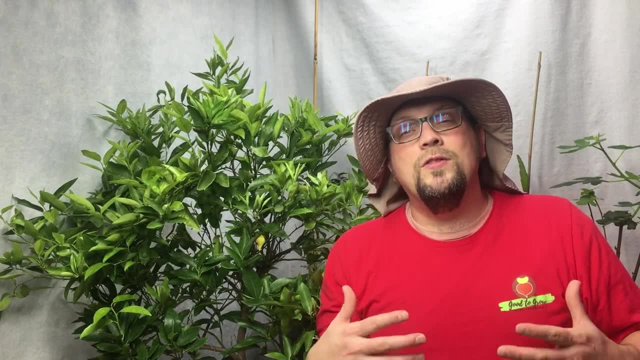 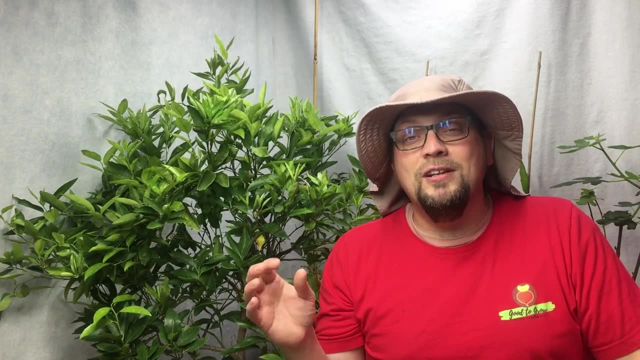 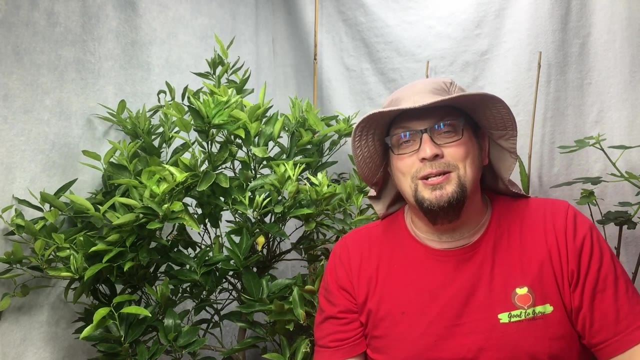 but that there's some excitement there around the food that they're taking in and that they're growing. You know one thing that you know about children: they definitely absorb what they hear from you and I guess that has its benefits, and it's also, you know, has its moments where it's a. 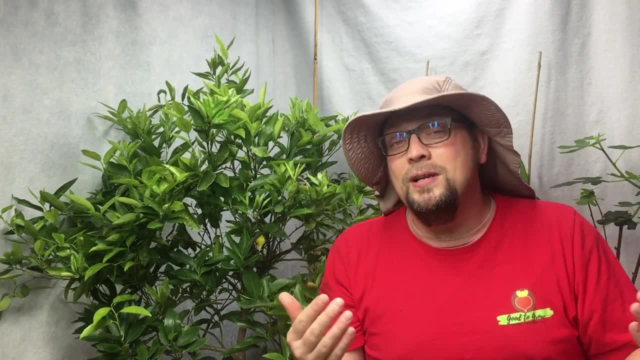 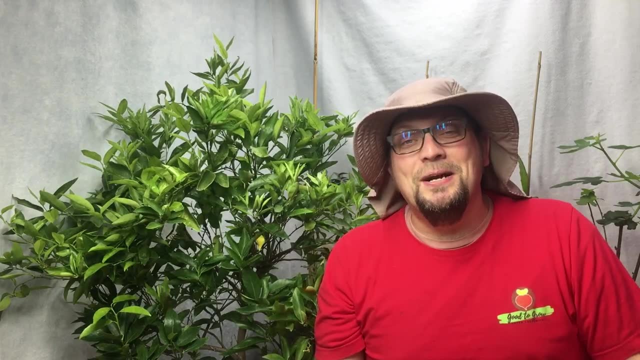 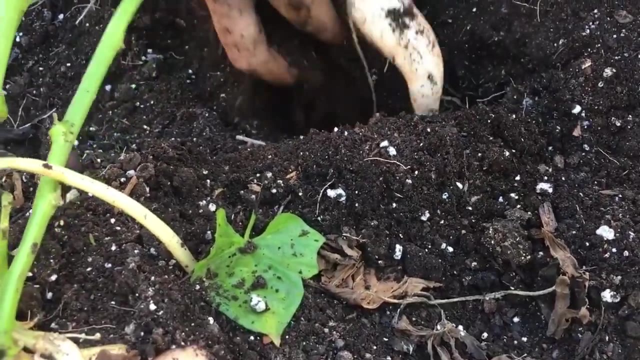 little bit more challenging, but one of the things- I can say it with complete pride in this statement- is listening to my daughter in some of her harvesting and how she's mirroring some of what we do here. Check this out, I'm digging way down, let's see. let's see what we got. We've got. 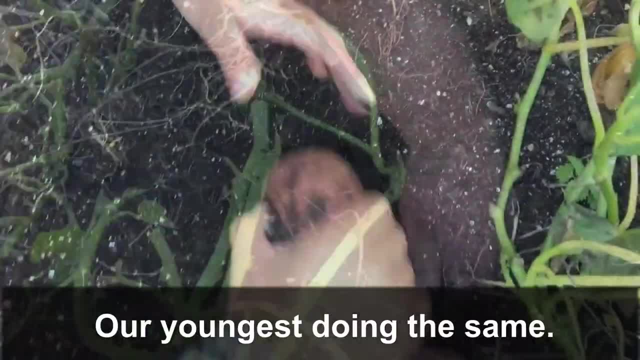 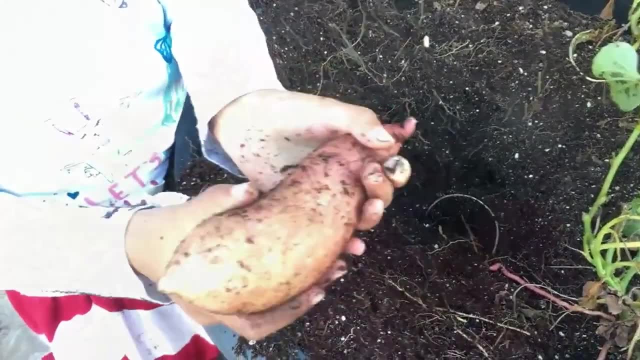 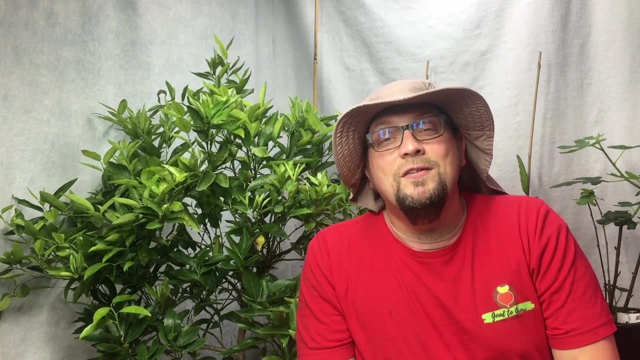 great sized sweet potatoes. what we got? Wow, This is a big, awesome. wow, look how big this is. Now, that was our youngest Yardner, but it's not just limited to the youngest, of course. we have both of our daughters involved in this process, and 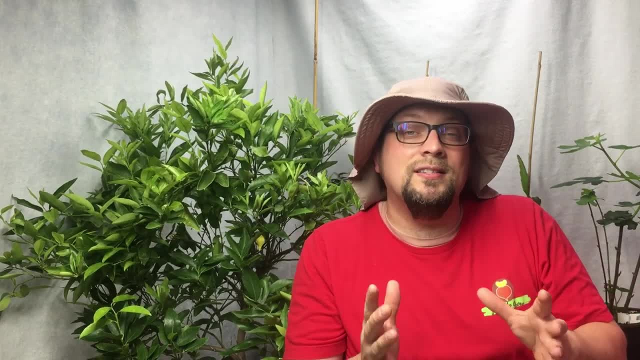 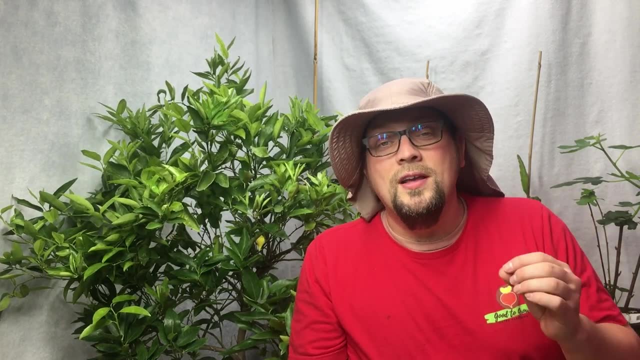 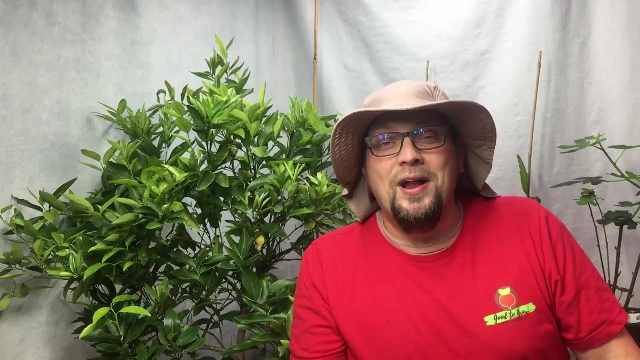 getting to see them out there harvest and express the knowledge that they have, that they've learned just from listening to us, is an incredibly rewarding and valuable experience. Here's an example of our oldest daughter Talking us through some of her harvesting of some radishes. smells so good, Smells like a fresh. 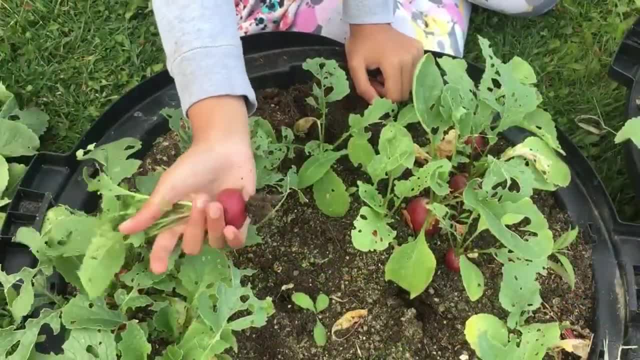 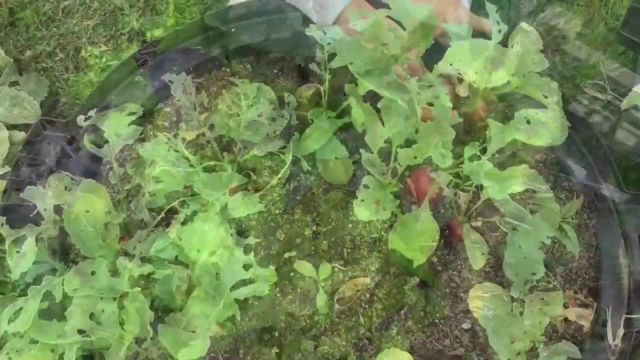 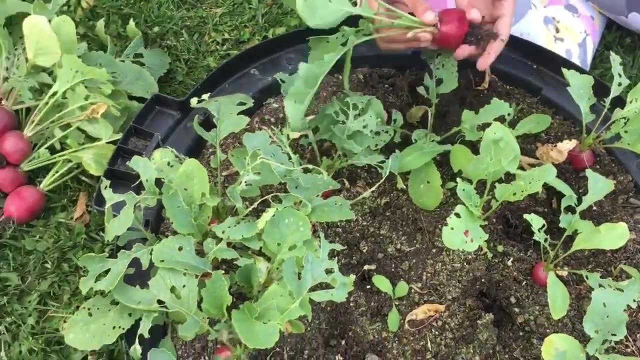 salad. This will go really well with what we got from our hay bale video. We got a whole bunch of good, fresh greens We have. one pound of radishes might be something we can go for, because radishes are not that big. They're the smaller variety of vegetable. 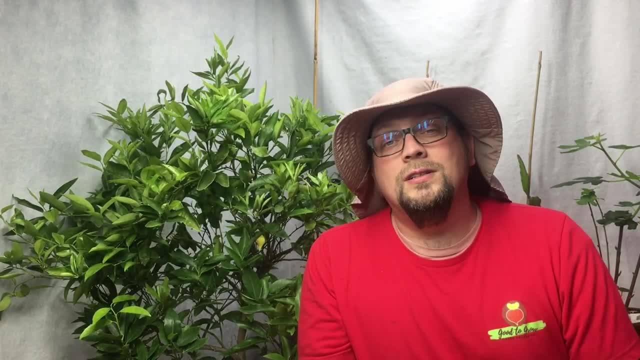 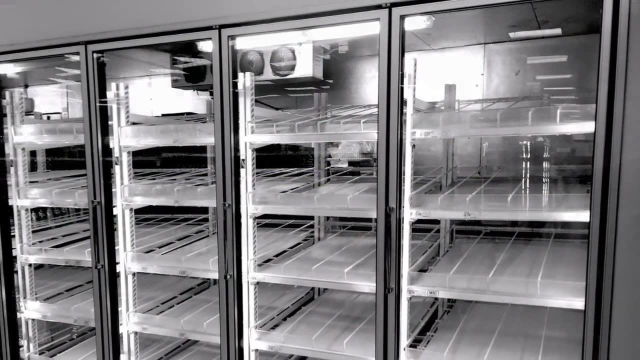 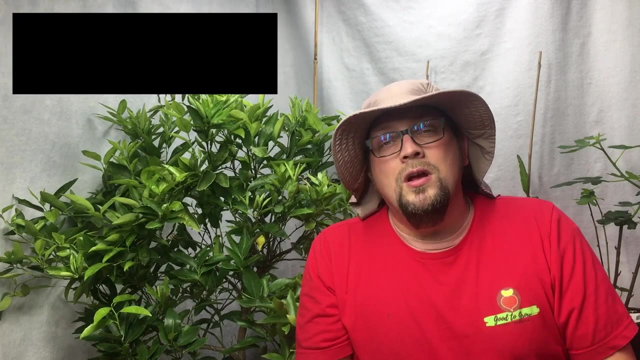 So what are we doing by getting our children involved in this process? Well, one thing's for sure: There's so much uncertainty when it comes to just the availability of food, when it comes to anything to do with the future, that it's our responsibility, from our point of view, our responsibility to pass on a skill to 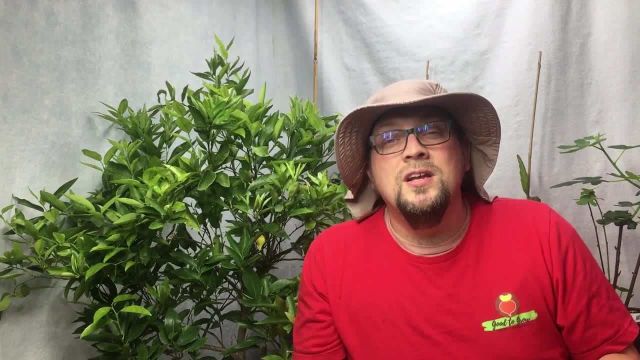 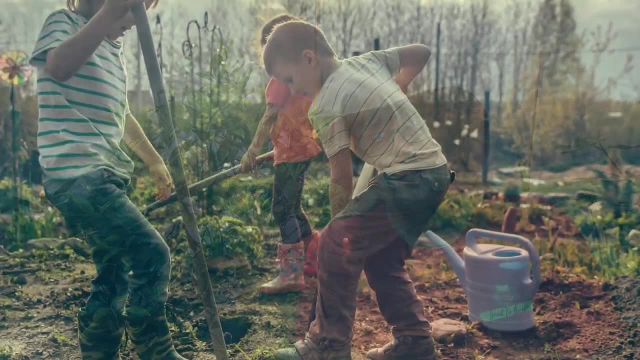 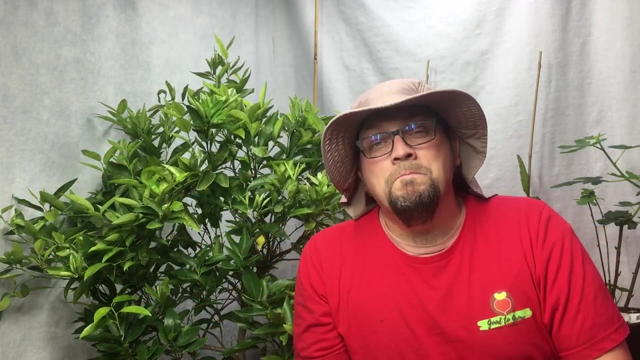 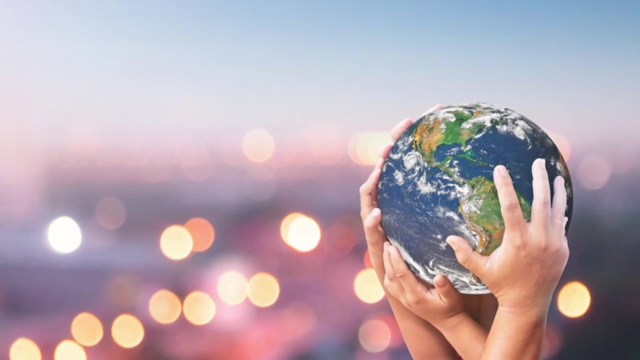 our children. that's going to benefit them, regardless of what's coming down the pipe in the future. and giving the ability to someone, or teaching someone the ability to garden and grow their own food, is such a liberating thing that we're doing. you know, our children have a responsibility to their community. they have a responsibility really to their entire. 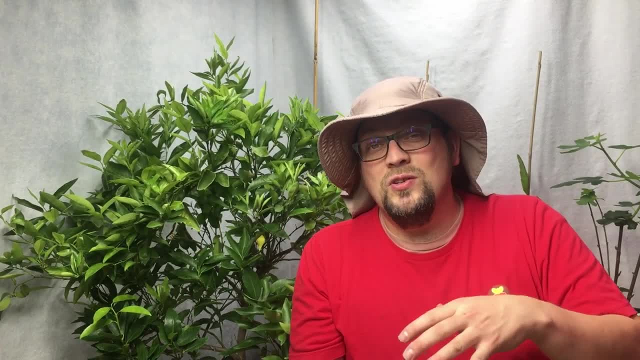 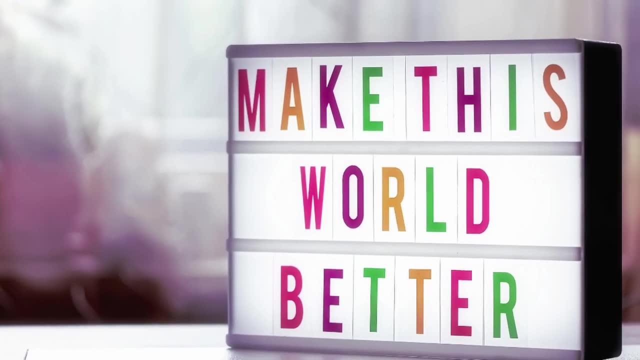 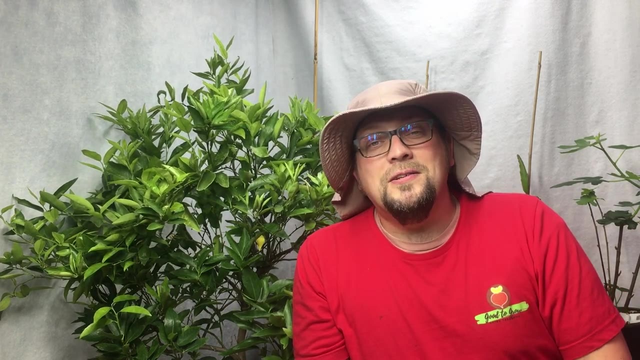 environment, and if we're able to add something to that so that they understand that responsibility and can also then build up or improve their surroundings, then what we're doing is creating a better future for them in many ways, and also, of course, for us. and the best part of it is- and I think about this from my days as a coach- I used to 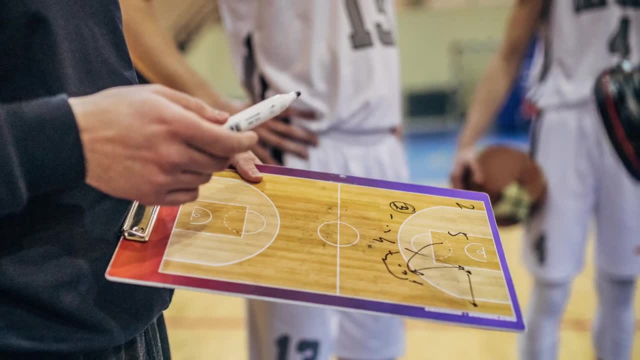 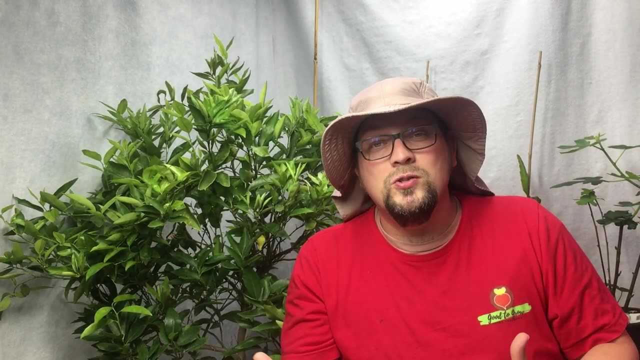 coach basketball. when I started coaching basketball, I got a lot better at basketball itself, because I was teaching the fundamentals of something to a bunch of children and also then practicing those fundamentals at the same time. well, let's take a look at gardening. I mean, we're learning, we're 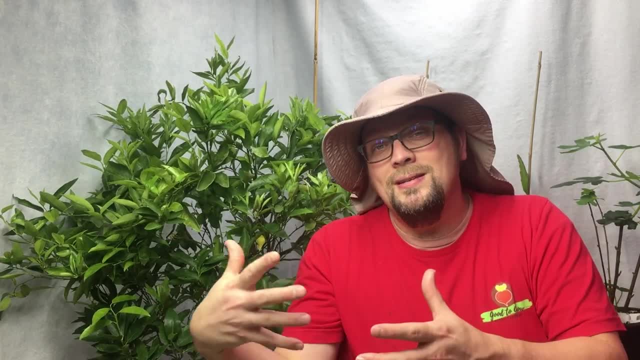 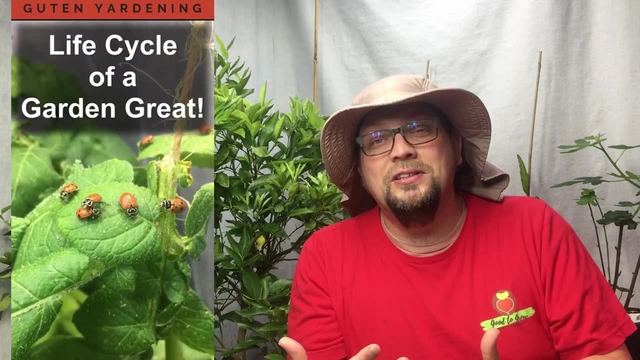 experimenting, we're experiencing new things and we're showing that and passing it on to our children. so at the same time, we're experiencing that same growth and what we're bringing to our children, our new experiences as well, that remove some of the fear that might be out of there. for example, when our daughter saw 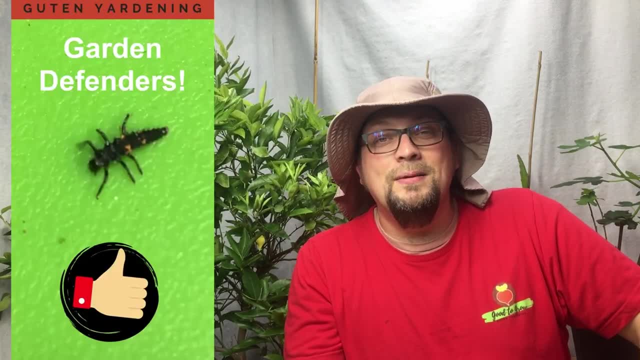 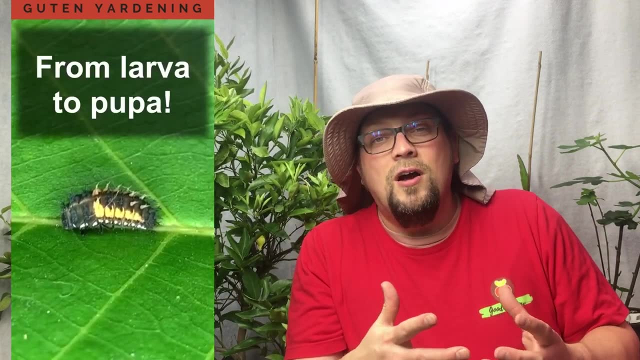 the ladybugs that we released in our indoor grow area for the first time. and that fear isn't there. there's the amazement, there's the understanding of the process, that life cycle of what we're doing, what we're bringing in and the purpose of some of these insects, and so, again, we're removing some of. 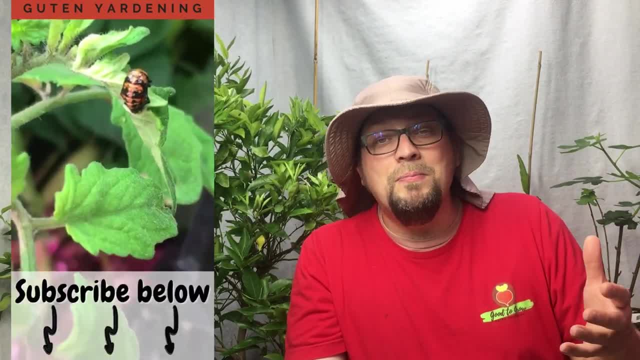 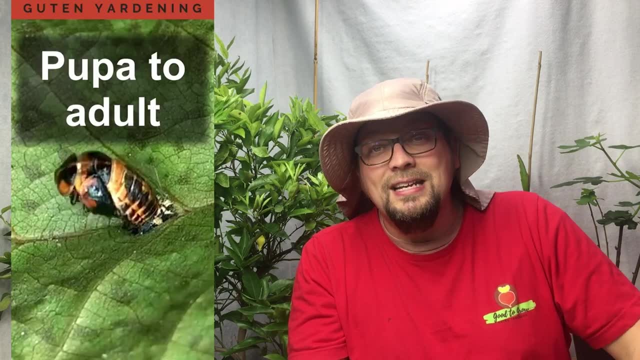 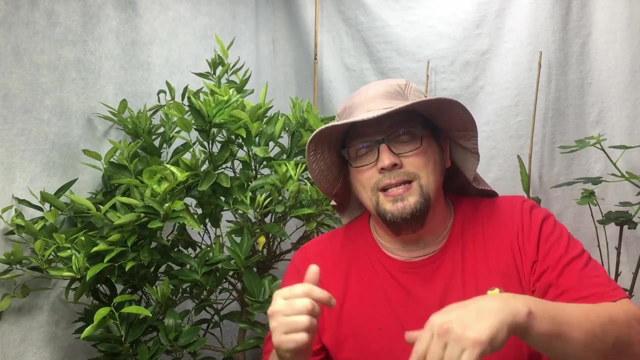 the unknowns from our children and providing them with, in my opinion, an excellent opportunity to gain knowledge in an area that's fundamentally important to what they need for the future. now, recently, I read a study- and this was a smaller study, I'll grant that, but I thought the study in general, which I'm going to link in the 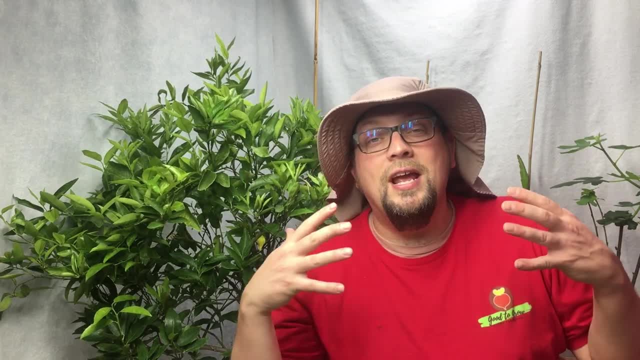 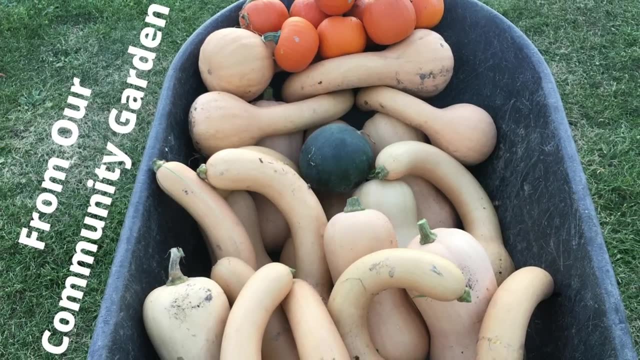 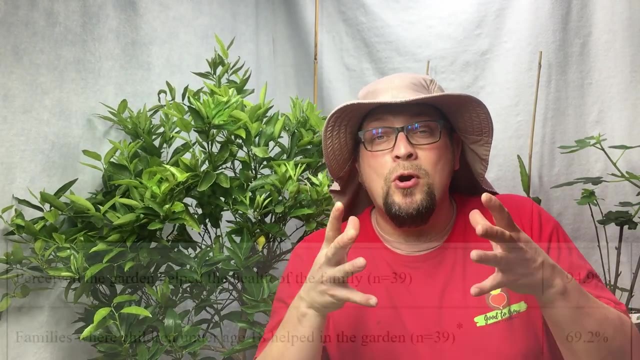 description showed a lot of promise, so the study was around a community garden, which is something that we take part in as well, in addition to our property. here we've done some community garden work, which is absolutely exceptional, and we enjoy that very much, and what they found in that study was that the people who were taking part in gardening in 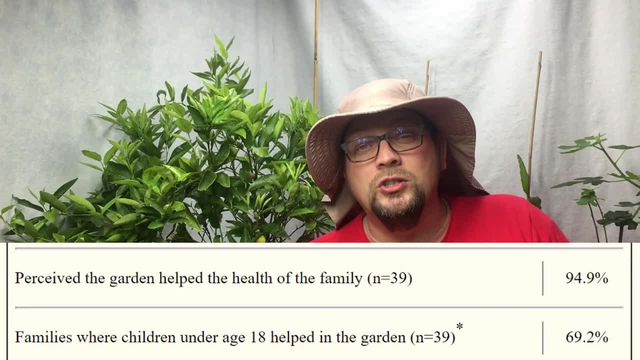 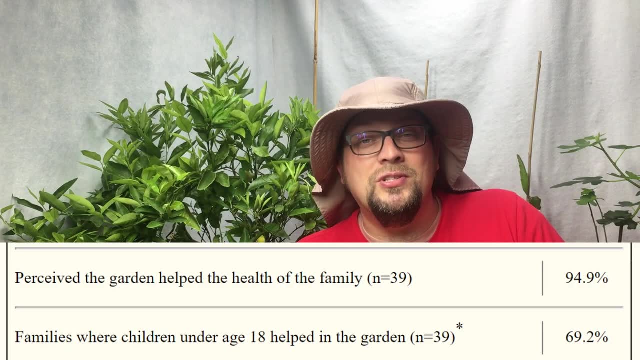 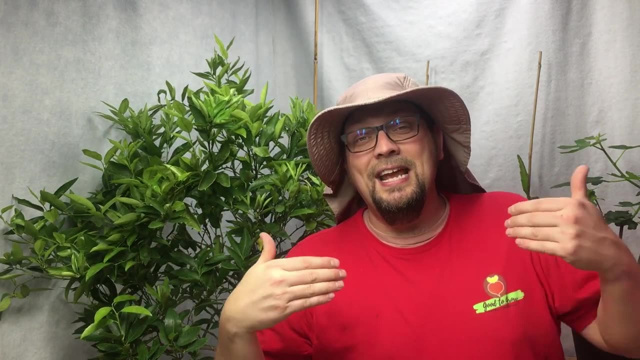 almost 70 percent of situations were involving their children ages 18 and under, and in over 90 percent of those situations, those individuals were encouraging other family members to take part and to take up gardening, so it's a very common experience for this to be a family affair. 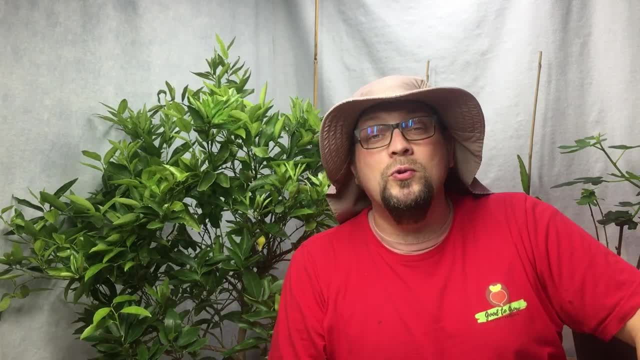 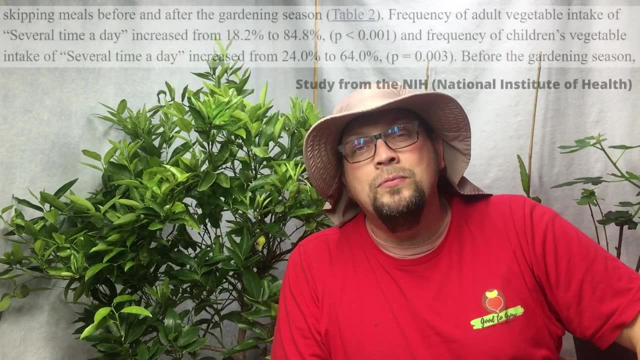 and so we're going to see how that goes along with you and have children doing that work with you and learning in that way. and you have the other thing that we found that I thought was incredible in that study: the children of those parents who were taking part in gardening were increasing their 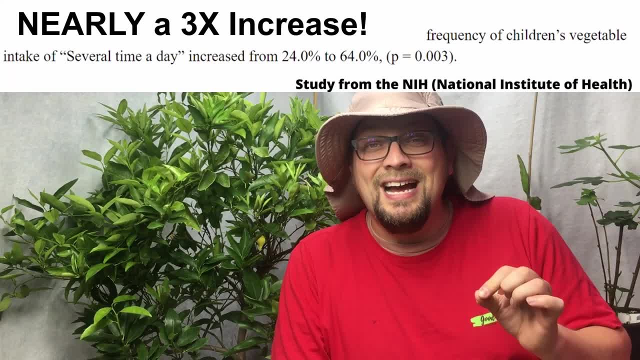 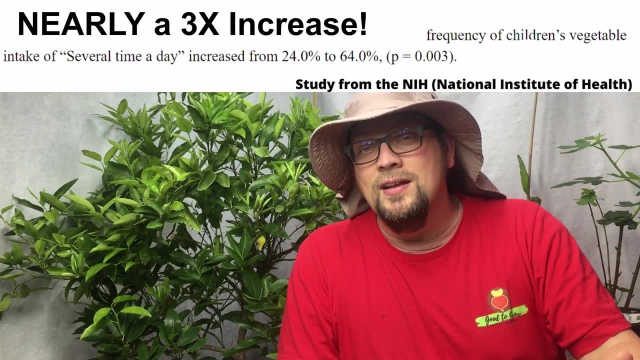 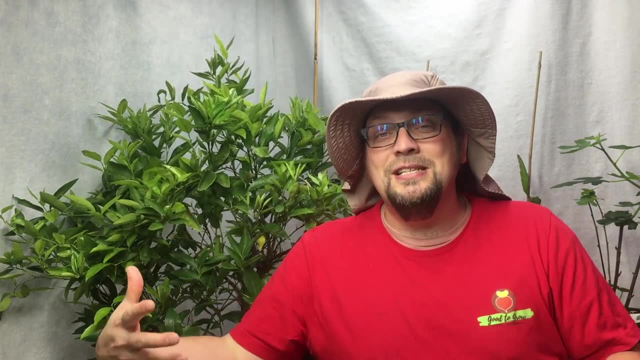 intake of fresh vegetables by three times. they were literally tripling their intake of healthy vegetables. so we're improving the diets of those children as well. so when we talk about this for our children, it's not just, oh, we're teaching them a new skill, we're also, hopefully, 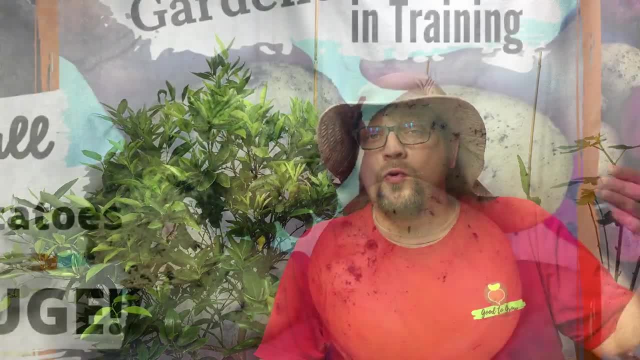 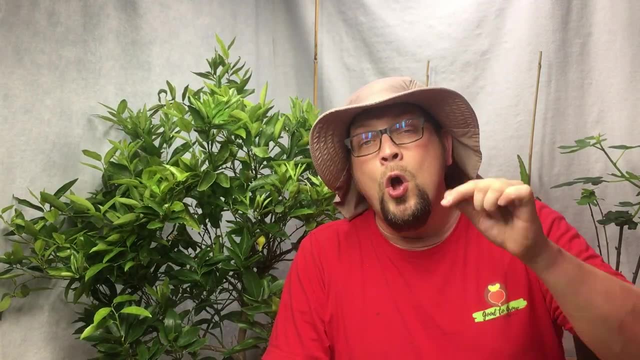 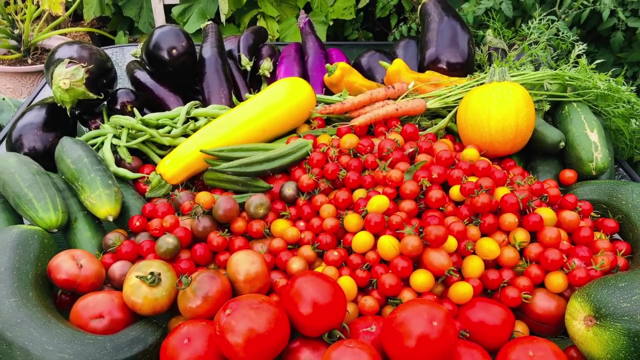 improving their diet. you know that's one of our goals here with our grow 365 challenge. we want to grow our own food 365 days a year and we want to be able to put those fresh veggies on our plates as frequently as we can, and as I was just eating some green beans from our garden this summer, this, 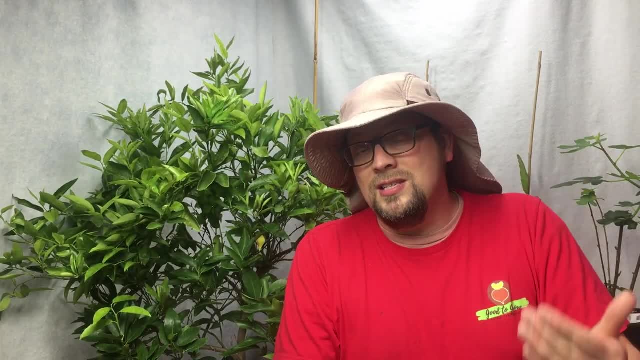 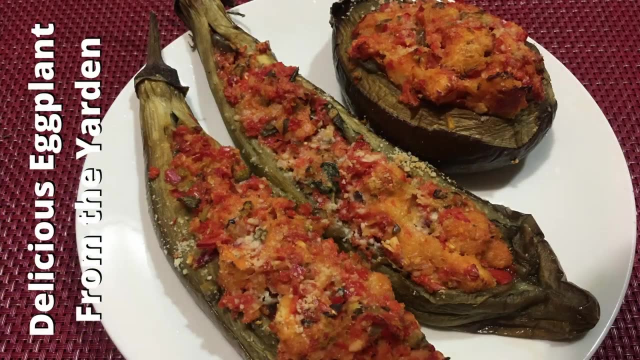 evening for dinner I was thinking, yeah, this is it. we're successfully doing this. we're including our children not just in the growing, in the harvesting process, but now we're producing food for them, putting it on the table. well, hopefully it's very clear to you that the family aspect of 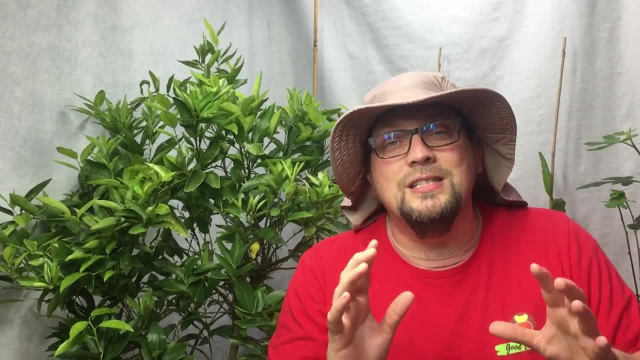 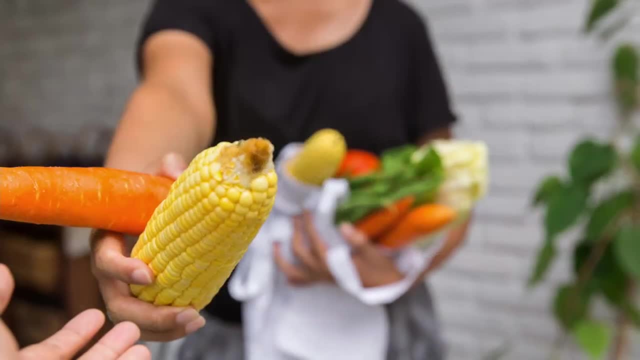 this our children. you know, not everybody has children. I completely get this, but the family aspect of this can go beyond that, of course, as well. you know, taking part in sharing the vegetables that you harvest with your community if you have excess, but also teaching those skills to our 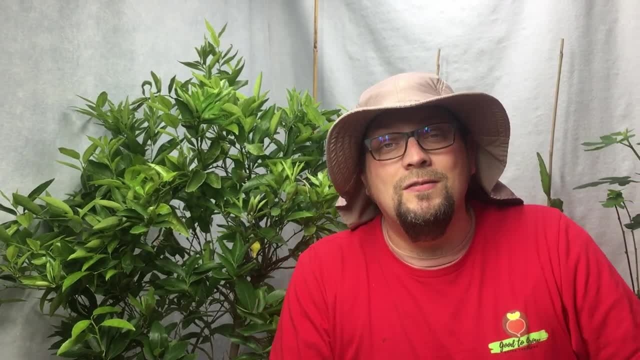 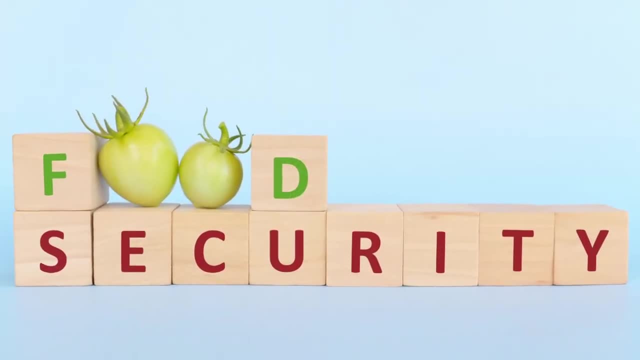 children as well. that idea of giving when you have to give. I mean that's a big part of what we're doing, and so we're here growing vegetables, we're gaining that food security and we're bringing our children right along with us on that process, and you know, 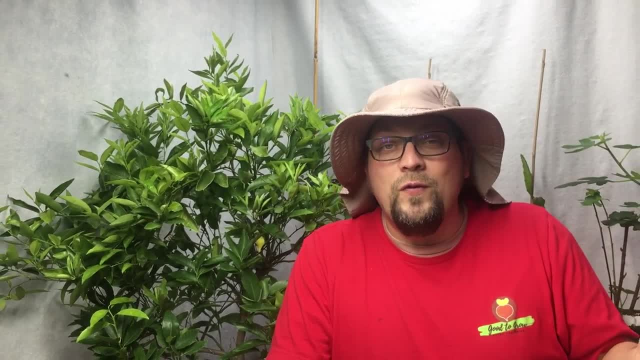 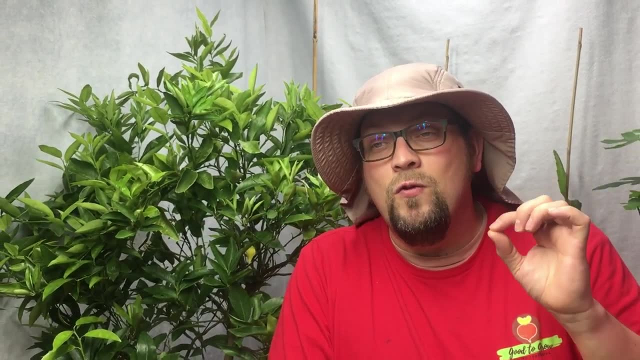 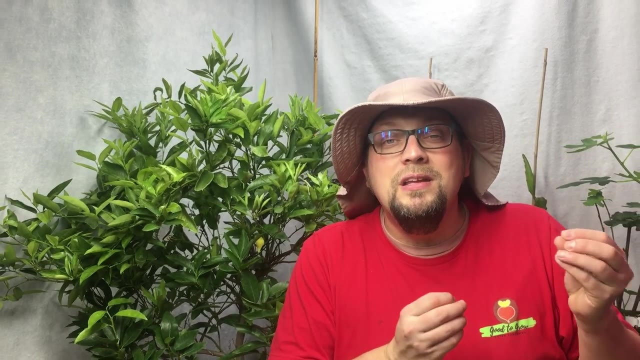 10, 15 years down the road, when they have their own families, when they're taking care of themselves. even if the gardening piece isn't something that they stick with for the short term, we know they'll have those skills in the long term and whatever they decide to do, they'll be. 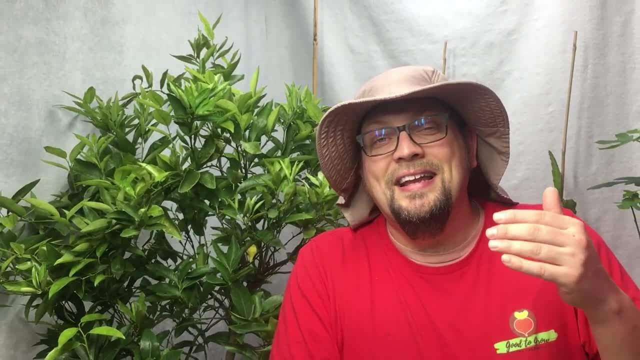 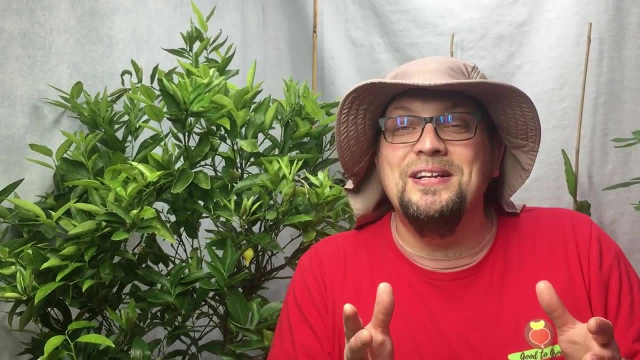 there for them first and foremost when it comes to gardening, is our family and taking care of them and teaching them the skills they need for future success. whether you are brand new to gardening or you've been doing this a very long time, we hope you can agree with us that this piece of it, this